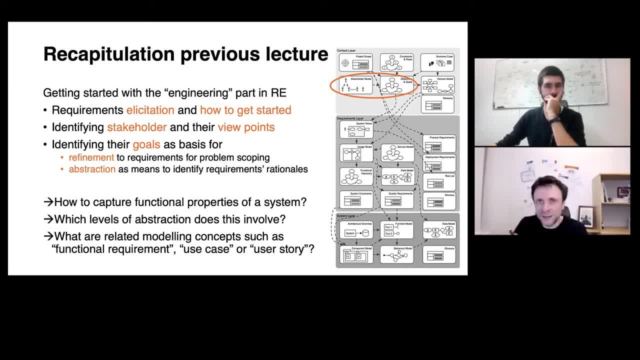 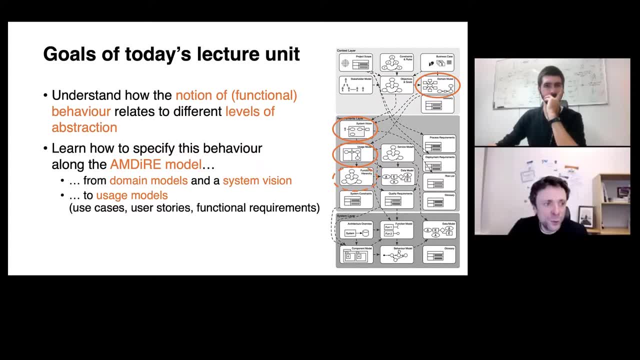 So an interesting topic. So an interesting topic And an interesting question is: how do these different concepts relate to each other? And this is exactly what is in the scope of today's lecture. We will be focusing on two different topics, not different related topics, one of them being we want to understand how the general notion of functional behavior relates to different levels of abstraction. 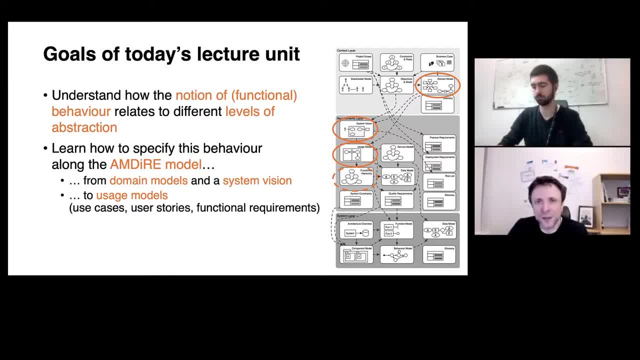 The ones we capture, And we want to address three relevant content items to specify this functional behavior, Namely being: the doping of the code function main model that captures the operational context of a software system. the system vision that captures a joint, unified vision about what is inside in our 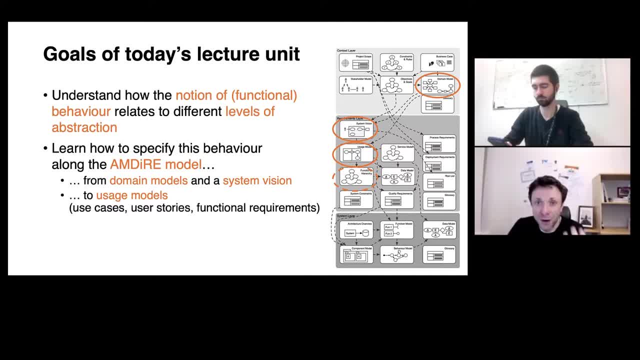 system and what is outside of our system. capturing the the boundaries of a software system and the major use cases I want to support with my software system and, finally, the usage model which serves as the content item for the functional requirements. capturing all these different complementary as we. 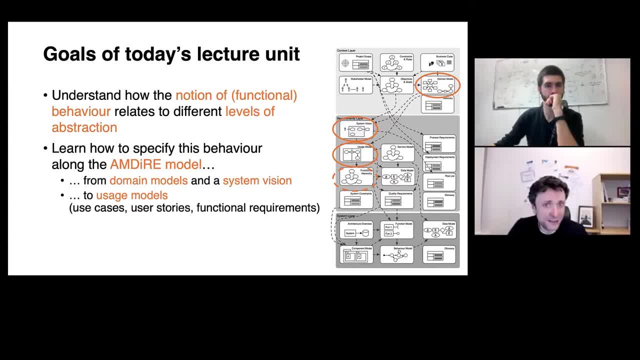 will see modeling concepts ranging from use cases and scenarios over user stories up to functional requirements. Now, before starting, maybe a small disclaimer. when it comes to the specification of functional behavior, the literature is literally full of different approaches, thousands of approaches of definitions, specifications of functional behavior. 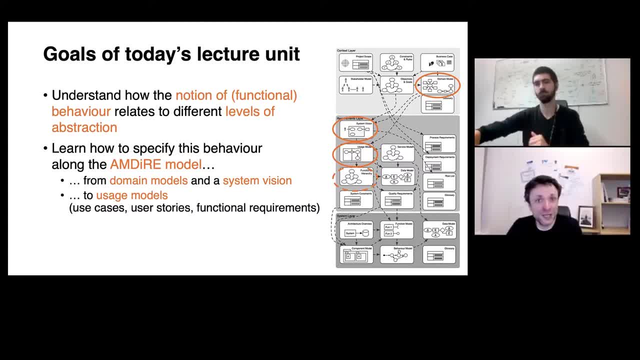 templates, representation techniques, notations, and so on and so forth. Now, the good news here- in contrast to non-functional requirements, as we will see, the good news is that there is a certain consensus, there's a certain agreement between all these different definitions, which gives us the privilege. 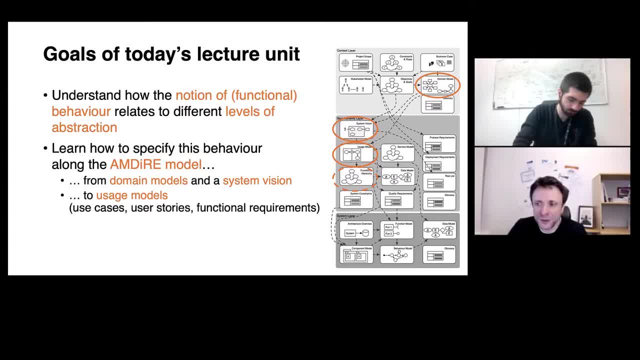 to take a more pragmatic perspective and concentrate really on the essential concepts, so how these different techniques relate to each other. So this does, as always, not replace the importance of having it done at least once, of having applied all these different techniques at least once, to learn what the different pitfalls might be, but also to learn what what might be. 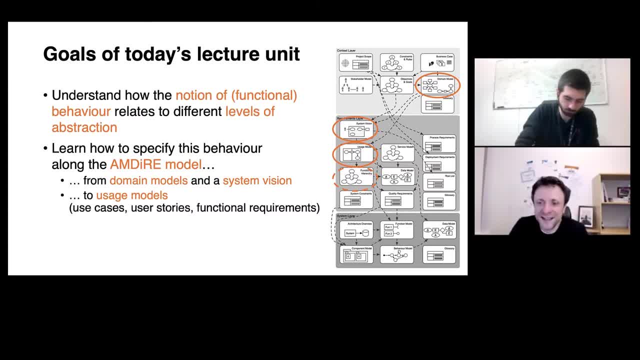 actually rather easy, maybe in contrast to a complex definition, and this is, as always, in scope of the hands-on sessions, the lab sessions and the and the project Q&A sessions. a second disclaimer I would like to make before I forget, As you will notice, not only today. 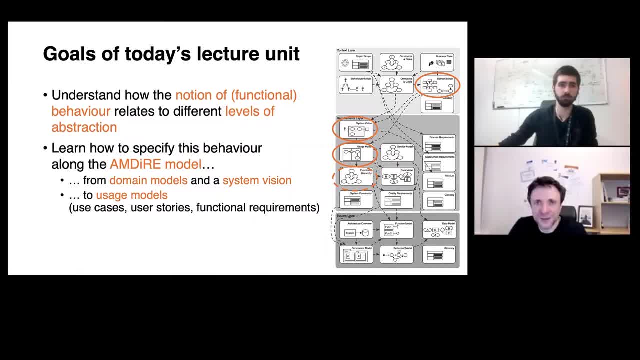 but also in the next lectures. there are some content items in the Amzire model we will not discuss, One example being a service model or a data model risk list. there are many. The reason is quite simple. The very idea is that I don't want to overwhelm you, but rather 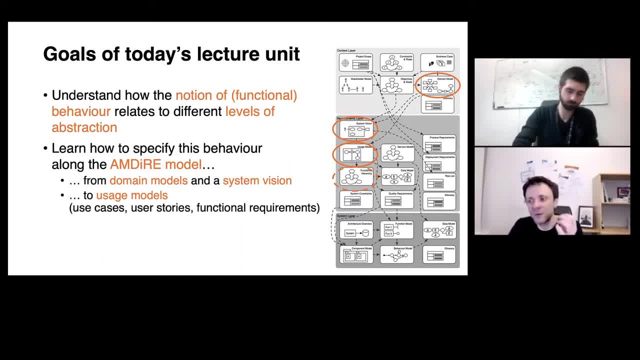 concentrate on the essence. So once we understood how to specify functional requirements, once we understood how to specify non-functional requirements, the rest comes easy And we can look all the information up, for example, how to specify a data model, because it's very much. 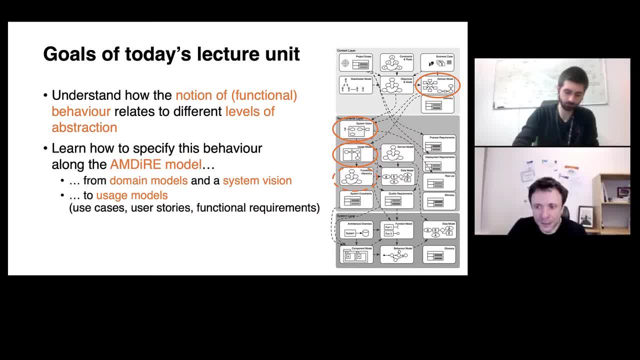 related to the notion of functional properties. Another reason is also that many of these content items are addressed typically in requirements engineering, but they are not really in scope of requirements engineering and therefore also out of scope of our course. These content items serve the transition. 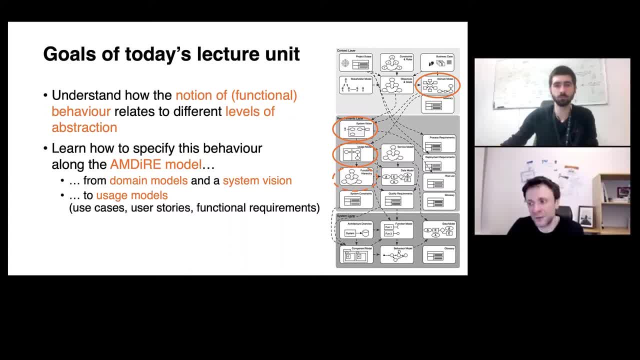 to the surrounding disciplines. The risk list, for example, serves the transition to risk management. The functional hierarchy serves the transition to architectural design. So you will find further readings related to those content items or extended slide sets that shall give you a big picture and shall illustrate also how all these topics that we discuss in this course, how these 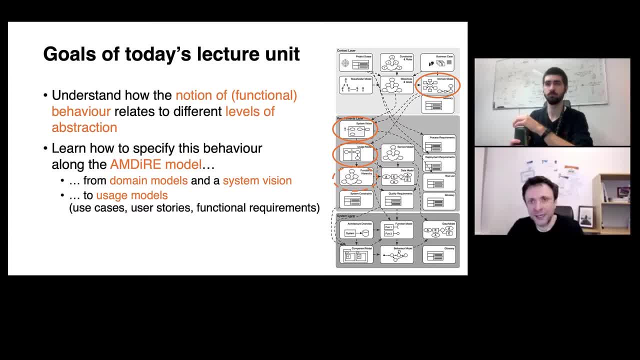 relate to the subsequent development phases, such as architectural design. This is for the curious reader under you, Which I know is every one of you, But nevertheless these are meant to capture more excursions so that you see also in other courses, how the things that we discuss in this course relate to those courses. 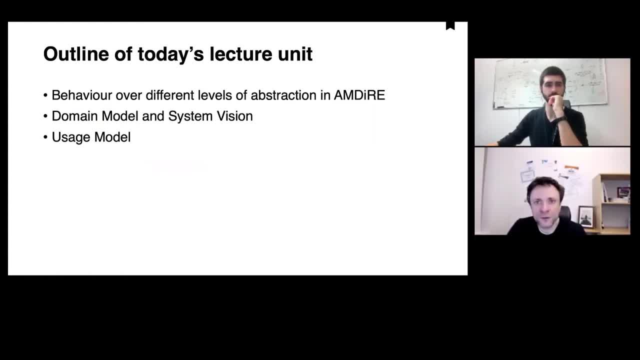 Now let's directly start. Today we'll focus on three topics. Number one: we will be discussing how this general notion of functional behavior relates to the different levels of abstraction and M-dia, before then discussing the single course. Number two: we will be looking at the content items, the domain model, the system vision and the usage model. 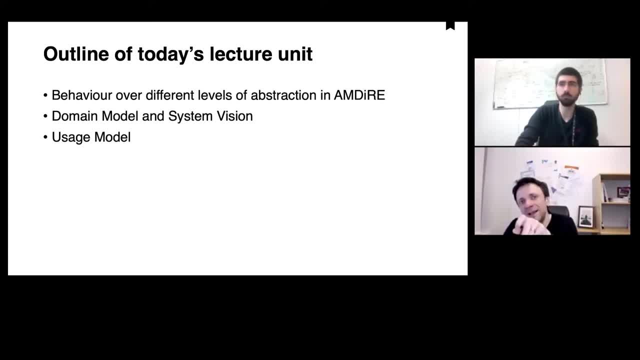 in more detail. This is exactly the point where we will be opening the little windows of our Advent Calendar and look inside these content items. So let's first discuss this general notion of functional behavior and how it relates to the different levels of abstraction. Here I will be iterating a couple of times through the very same levels of abstraction. 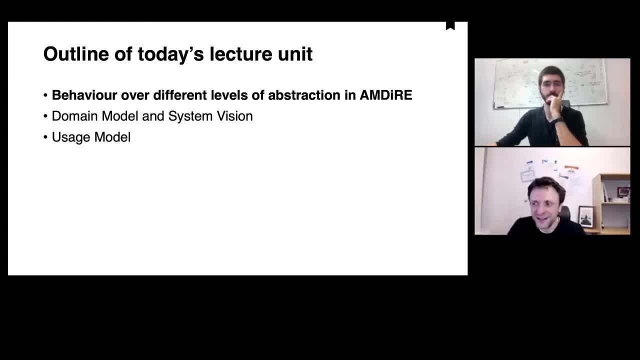 and I might, to some extent, maybe sound a little bit like a preacher or a politician, I don't know. But rest assured, the idea is not to turn some baseless claims into truth, into facts, but rather than giving you different perspectives on the very same concepts. 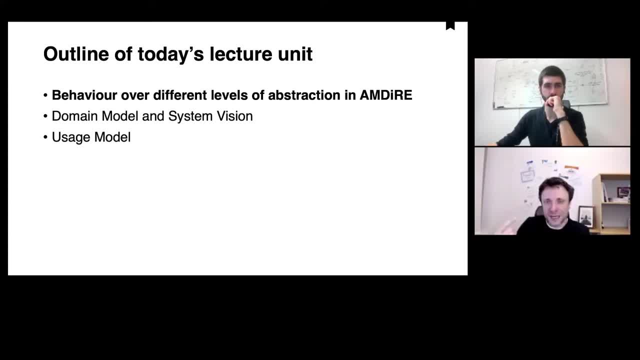 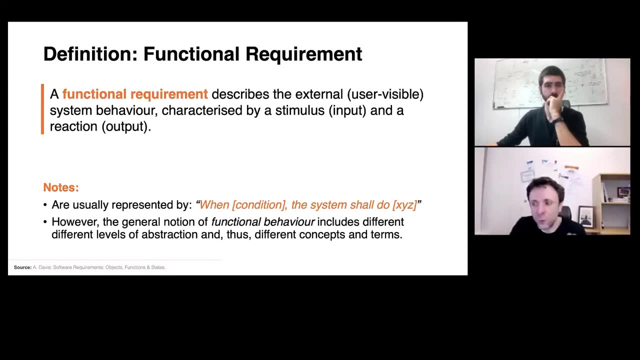 so that you can wrap your head around this. So give it some time, give me some patience and you will see how straightforward actually functional modeling intends to be. Now let's directly start by jumping into the cold water and discussing what is a functional 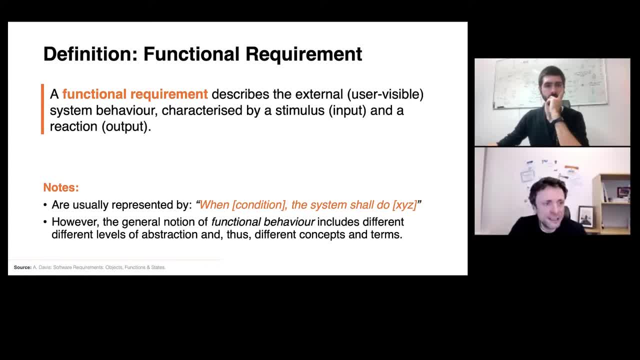 requirement. So what you can see here is the definition by Davis, which is one of my favorite definitions because it's very straightforward and up to the point. He says that a functional requirement describes the external, user-visible black box behavior on a software system characterized. 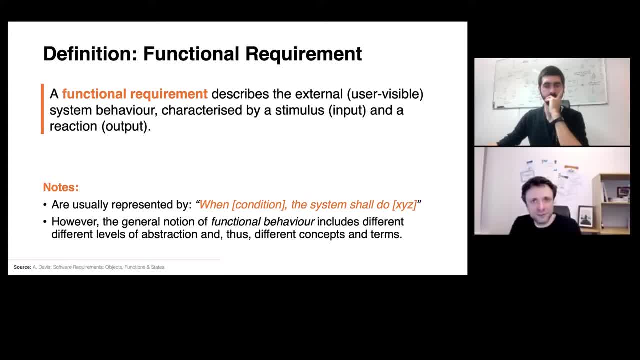 by a stimulus, by an input and a reaction, a response or an output. And it's simple as that. It's an external perspective on a mathematical function. I throw something into that function, the function processes something and it gives an output In terms of requirements. engineering. 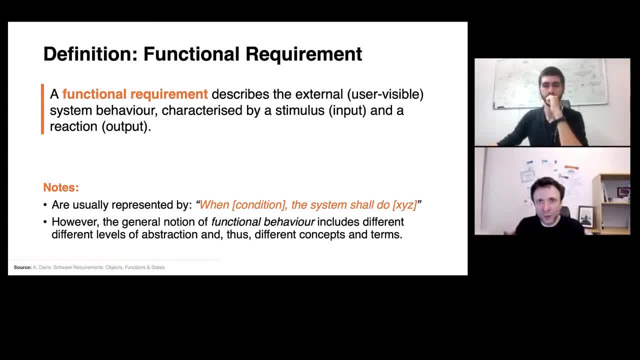 I specify what reaction I want to perceive from the software system when giving it a stimulus. So I want to describe essentially what reaction I, as an external actor, expect from the software system. It can be a human being, but also an external system. 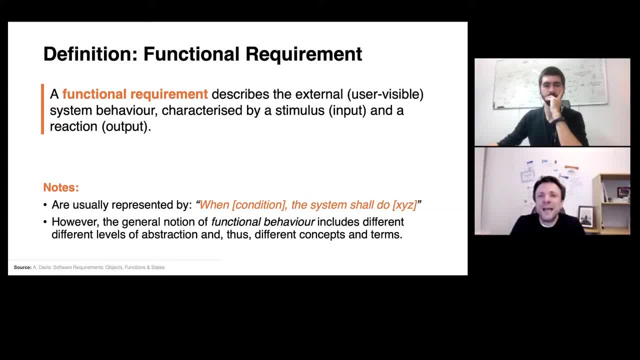 What I, as an external actor, expect from the software system when interacting with that software system. So typically you find functional requirements in the form as represented on the bottom of the slide, and natural language specifications following certain patterns, and one form or the other saying when there's a certain condition, when I deliver a certain input. 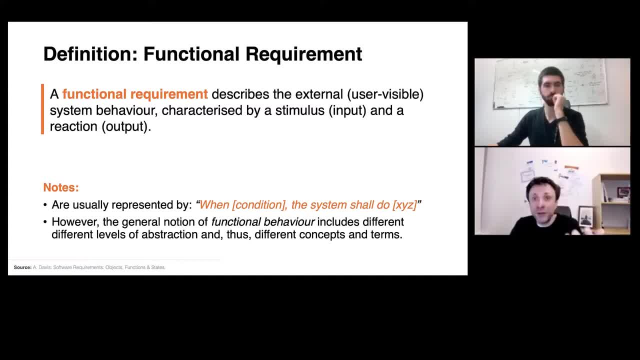 when I press a button or when I use my search engine, when I type in a search query, I want the system to deliver a certain response following certain characteristics, without restriction, restricting the solution space, without saying how exactly it should process my input. So this is the very essence of a functional requirement, but there's much more. 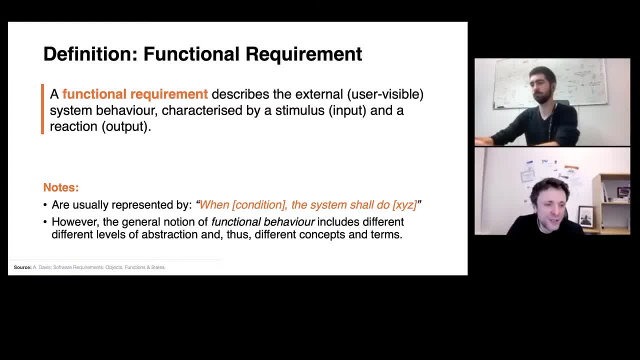 to it. And one thing to understand is that this very general notion of functional behavior includes different levels of abstraction, some of which don't even consider a software system at all. So always keep in mind: software is built by humans, for humans and those humans who intend to be supported by a future software system. 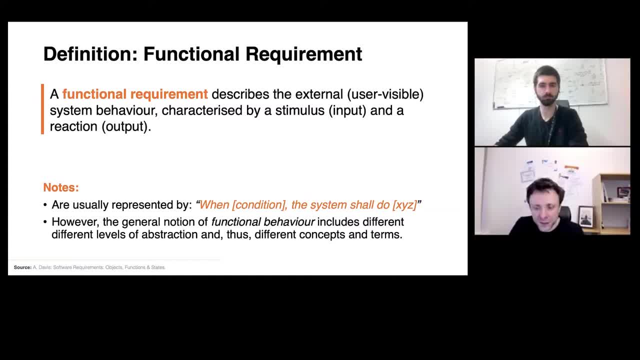 they operate in a specific context, And this context is typically characterized by workflows, by tasks that they want to achieve, by procedures that they want to follow in a business, for example. And one specific task in requirements engineering is to understand that context and to infer requirements towards a software system so that this software system 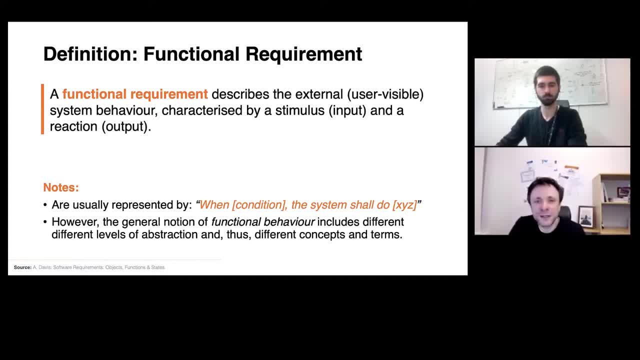 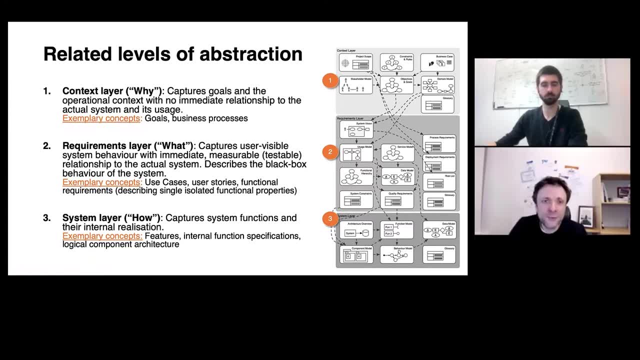 fits that context, Which brings me to the different levels of abstraction. Now, the levels of abstraction that you can see here, you know already. So we distinguish the context layer that gives answers to the why question. So why do we need something? We have the requirements. 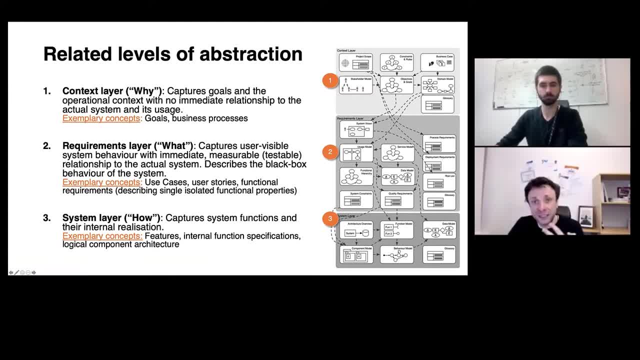 layer that specifies user visible characteristics of a software system. So what should be done? We have the system layer that specifies how it will be implemented, the glass box view on a software system. So in the context layer we capture typically the goals and the operational. 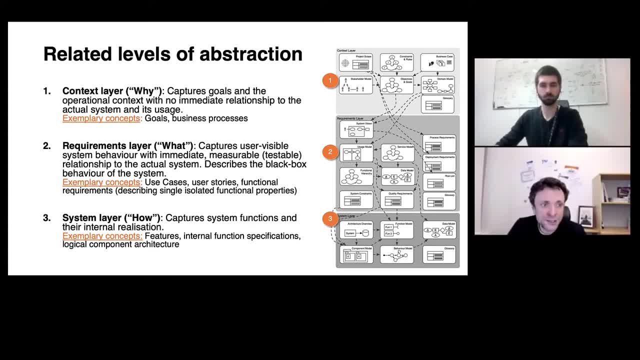 context, with no immediate relationship to the actual system and its usage. So what we do here is we capture our understanding of the real life operational environment and all those tasks that need to be accomplished when making use of a software system. So, for example, all those tasks that I might find in a banking sector- Banking processes, for example. 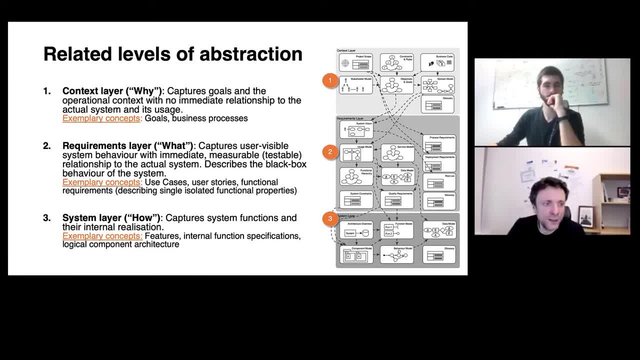 when opening a bank account or when registering a user. Now in the requirements layer we capture the user visible external black box perspective on the system behavior with immediate, measurable, that is, testable, relationships to the actual system. So here I specify how I as an end user, 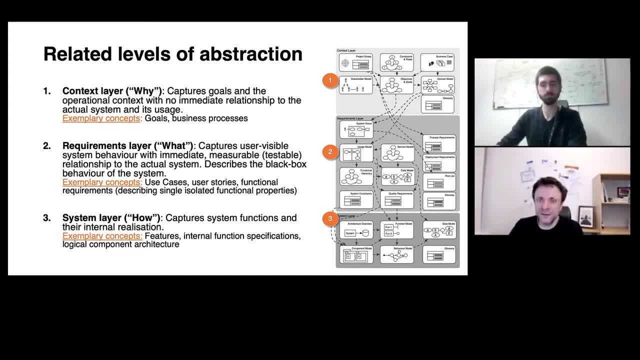 intend to interact with the software system in context of my tasks, in order to accomplish those tasks. In the system layer then I capture the system functions and the internal realization. So here is when I describe how my software system should be realized in order to support those intended interactions. Now a couple of other terms that you might find in. 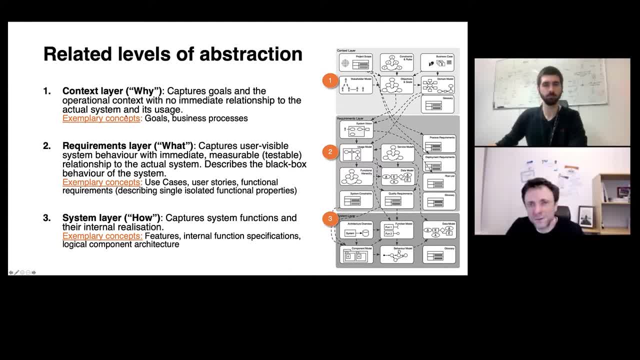 literature is that the context layer is often characterized as business requirements because very often we describe the operational business world, the perspective on the workflows, on the tasks For the requirements layer. very often the term user requirements is used because we describe user visible characteristics of a software system And 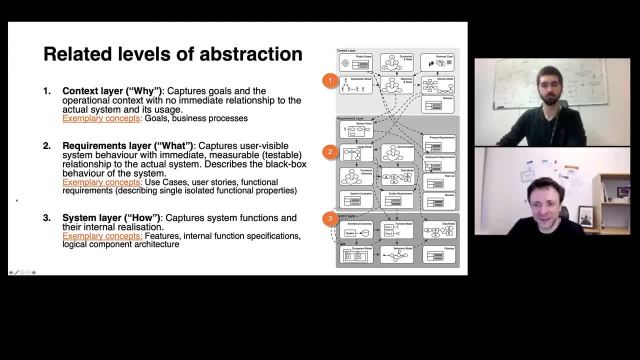 the system layer is very often called system requirements, because we discuss here the what at a system level. Needless to say, I'm not a big fan of those terms, because the system level requirements or system requirements somehow suggest that we are still talking about requirements, engineering, when in fact we are talking about the solution, space and rather design activities. 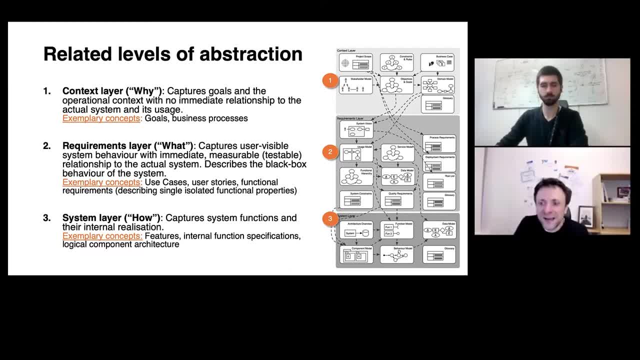 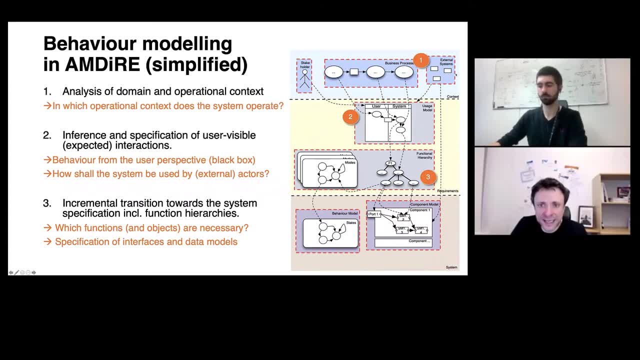 Now let's go through this picture again, but this time we will put focus on what we actually do and the underlying modeling concepts. Now, here you can see again the context layer, the requirements layer and the system layer. Now, in a first step, I tend to analyze the domain in the operational 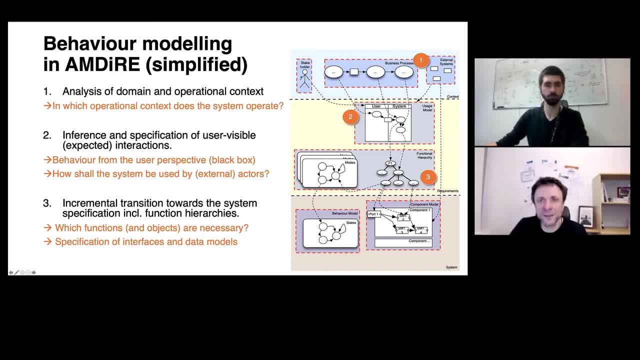 context, I want to understand what the typical workflows are, what the typical tasks are, which stakeholders are involved, what the goals might be, but also what the more operational environment like, what other external systems that might or may not maybe play a role in that system. 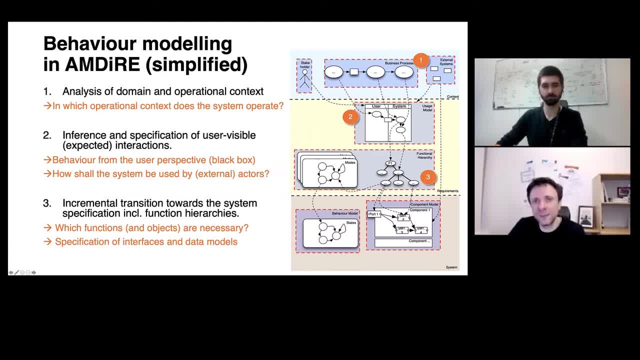 Now, here we concentrate on really understanding what the typical workflows are, For example when opening a bank account. In a second step, I want to infer and specify the user visible behavior in the form of requirements, in our case in the form of functional requirements, and to this end, I'm 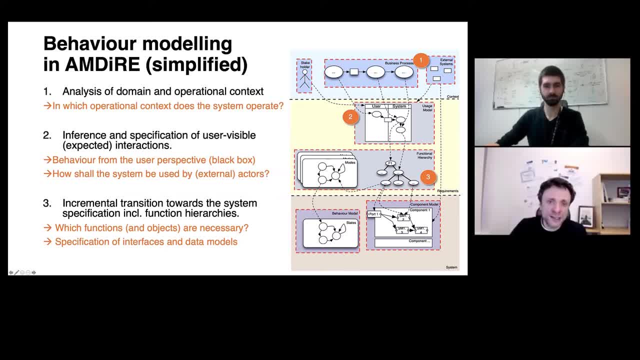 relying on what we call the usage model. Here I want to understand how I, as an end-user, intend to interact with a software system in order to realize certain tasks in a system-supported manner, Which means that for some of the tasks, I decide that maybe those tasks remain the responsibility of an 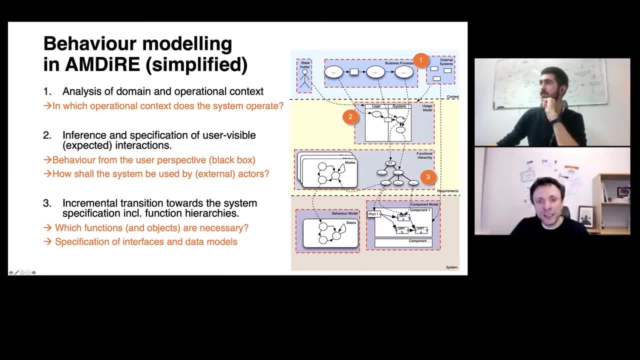 end-user. Other tasks, however, might be in scope of a software system. So, for example, when I try to authenticate or to verify my user identity in a bank, I might process some information, exchange some information and my usage model here. 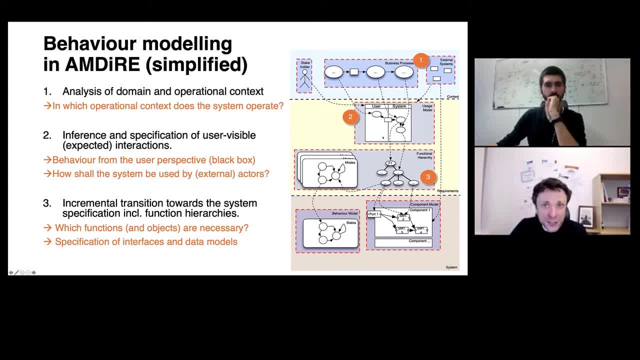 exemplary, visualized with an interaction diagram. here I specify how I can do this with a software system. So I enter certain credentials, maybe, and the system processes those credentials. In a third step I prepare for the transition to the solution design, to the solution. 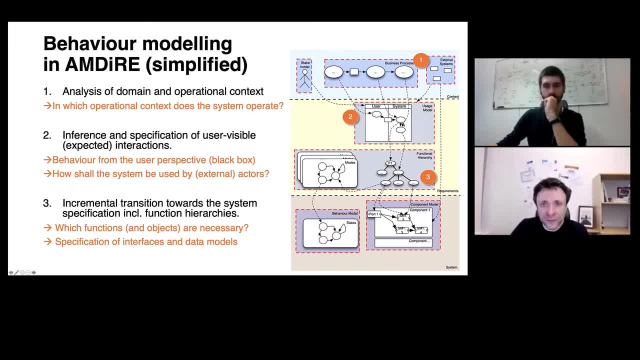 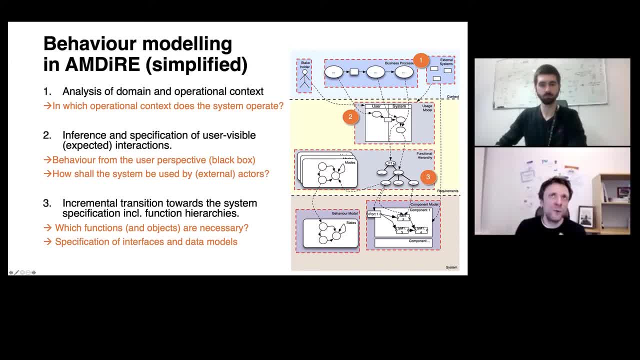 functional hierarchy. So at this stage I decide which sub functions do I need, what structure would I like to include? which means what could the interfaces be that I might offer with my software system? how can I further refine it into a logical and, later on, a technical component, architecture and 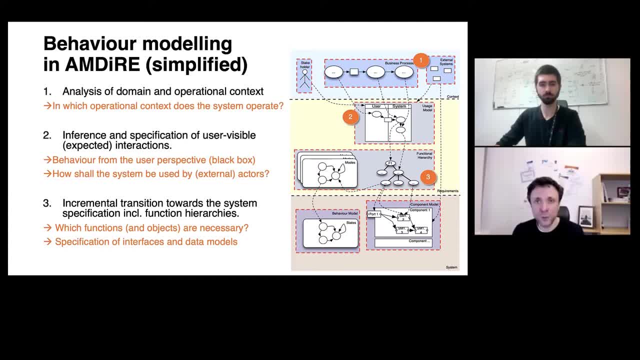 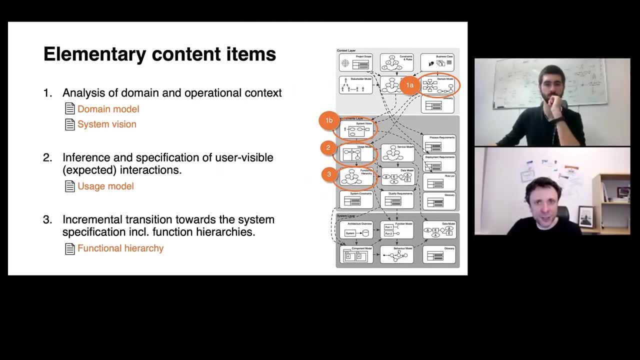 so on and so forth. So this is clearly in scope of design activities. Now let's go through this again, and this time we focus on the content items of M-Dial. So when the first step, when I analyze my domain in the operational context, when I 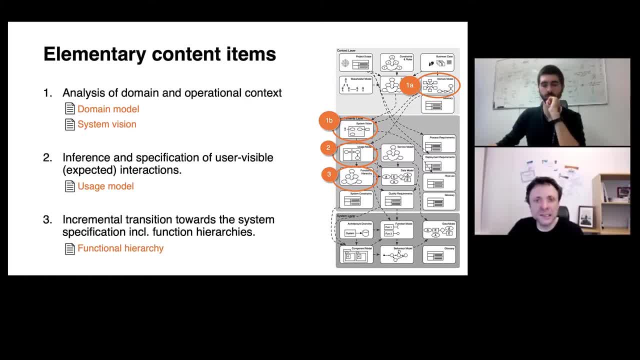 want to understand what the real-life environment is of my future software system, I specify the domain model. Now, the domain model captures my understanding of the operational context of my software system, represented by different views I can take on the domain. One is a workflow view, another one is a more static view on the 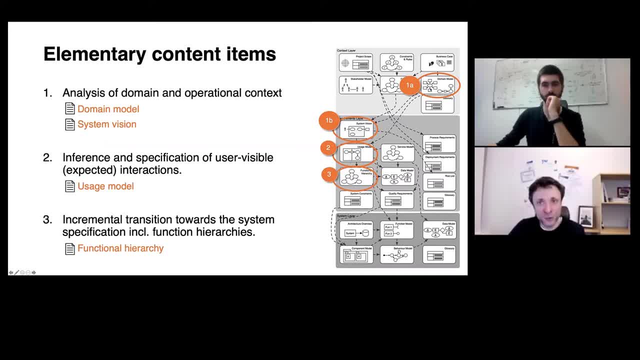 objects that might be important in the domain. I will show you this in more detail later. In a second step, I infer what we call the system vision. The system vision is the means for communication and for scoping, because it defines what the boundaries of my software system are and what the major 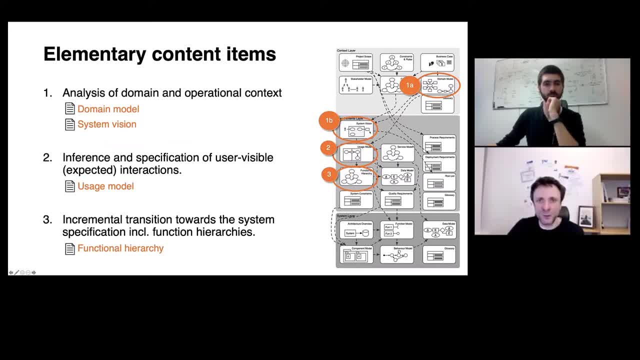 use cases will be that I want to support with my software system. In a second step. I define what the boundaries of my software system are and what the major use cases will be that I want to support with my software system In a second step. 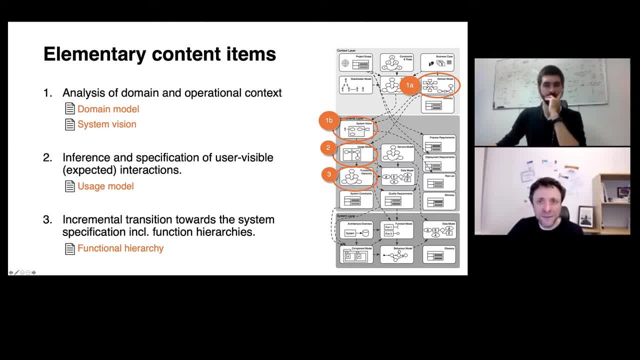 I infer and specify the user visible behavior, which means that for every use case that I indicate in my system vision, I infer a usage model in the form of interaction scenarios that captures how I, as an end-user, intend to interact with my software system. And in the last step, I identify those system-sided actions. 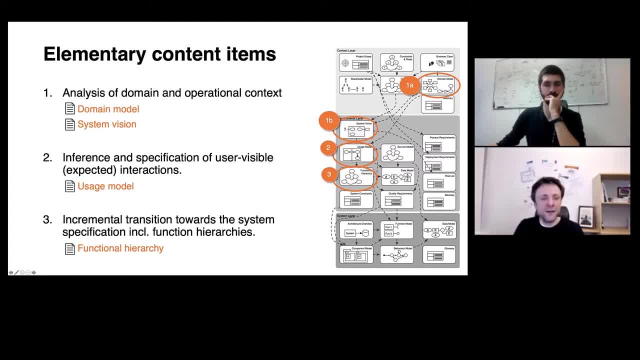 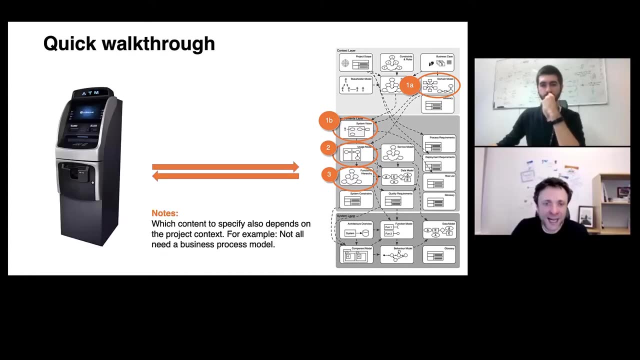 those system-sided functions and refine them further as a means to move on to the solution space. Let's go through this once more, but this time with a little bit more detail. we will be looking into the actual content items And again we will be relying on our banking example, using our beloved ATM. 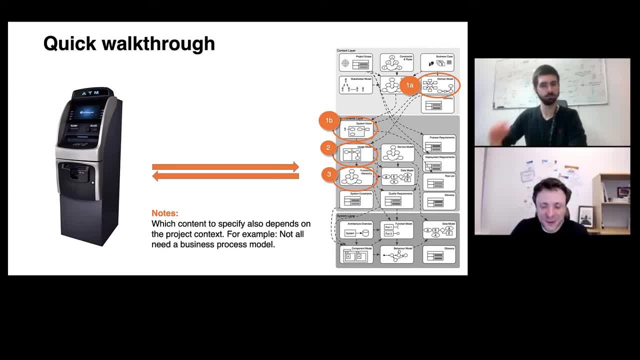 As always, always keep in mind that how exactly we specify our contents, our content items, but also what notation we want we might want to use, very much depends on the project context. So keep in mind we will will be talking about business processes, but not all systems need an understanding of business. 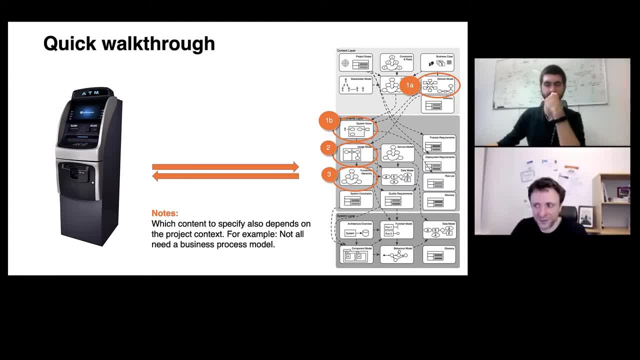 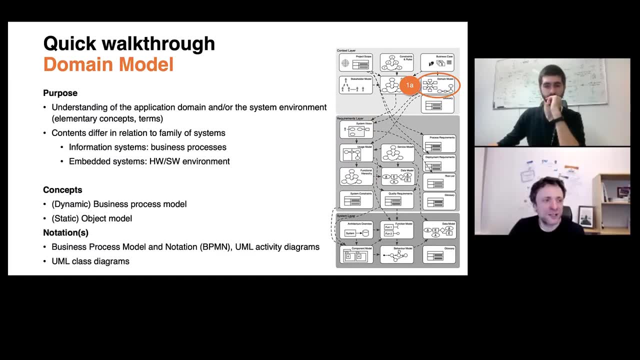 processes. Some of them don't even have business processes. but more on this later. Now let's start again with the domain model. As I said, the domain model captures our understanding of the application domain and the system environment. So here I want to capture what the real life operational 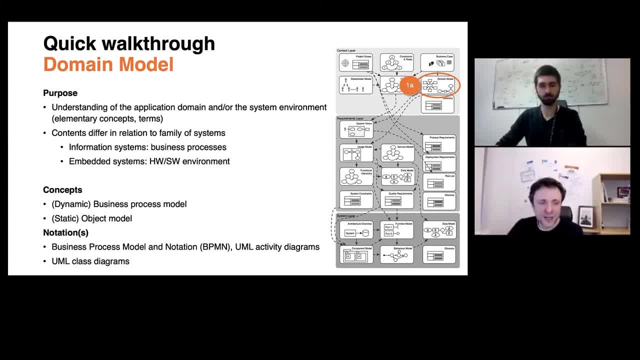 environment of my system under consideration is- and I can do this by capturing two perspectives, and which perspectives I take very much depends on the application domain and, more importantly, in the underlying family of systems. So typically I focus on workflows, on tasks that human stakeholders might want to perform and which human stakeholders might want to have in a system. 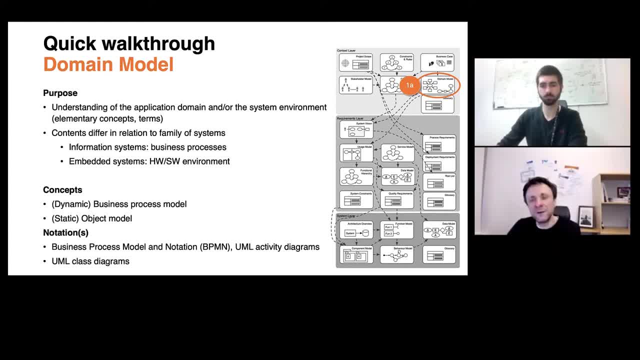 supported manner. So a classic example for this are information processing systems or business information systems. This is what I typically found in domains that are heavily dictated by workflows, Ways of working, tasks that I want to achieve- An app, for example, I want to achieve a certain 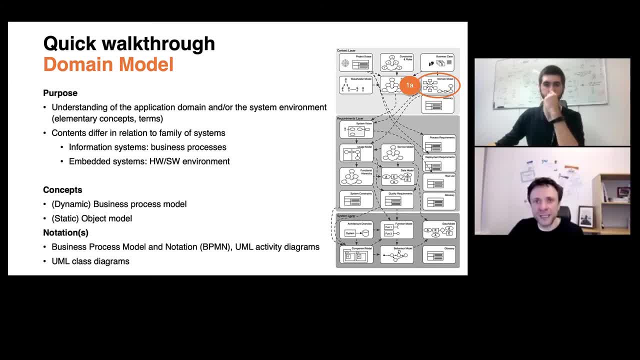 task with my app, and this is typically characterized by these more dynamic perspectives that I can take on my domain. The other perspective that I can take is a more static perspective, where I try to understand what the operational environment is, what the objects are that are processed. Both 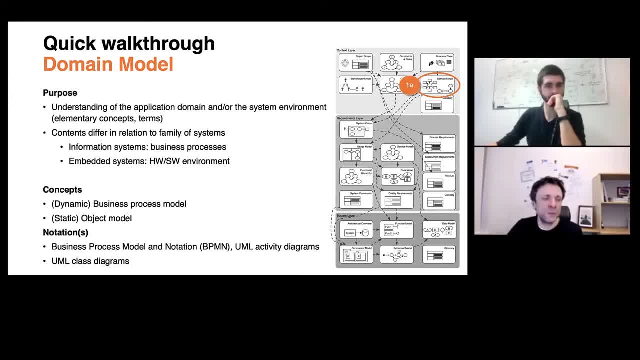 perspectives are rather complementary, but the second one tends to be more important in domains that are more dominated by a hardware view and a software view, So embedded reactive systems, for example, in the automotive sector, where many of my software systems don't interact with human beings, but rather with purely external systems. Now, what you can see here is one example. 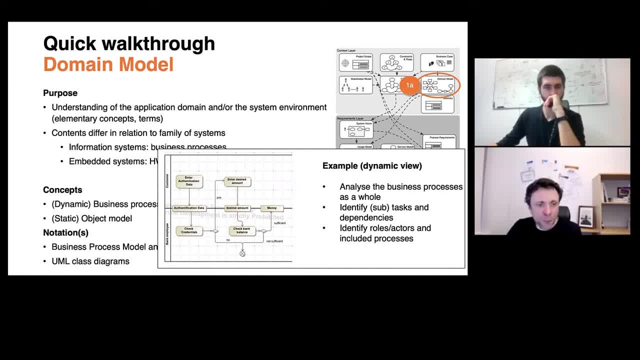 for a dynamic view captured by a business process modeling notation. What exactly we do here is not that important, but take away one thing, that is, that at this level the application is more dynamic. I don't specify how I intend to interact with the software system, but rather I really want. 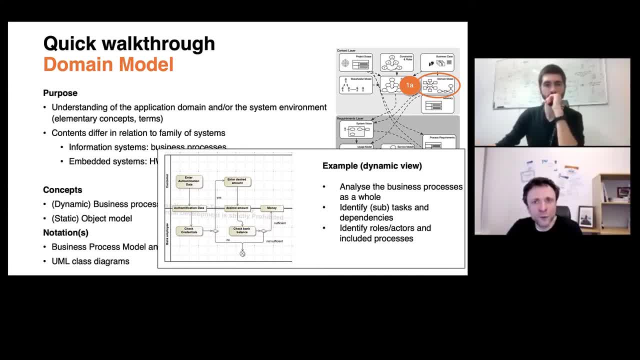 to understand only what the generic workflows are in my domain. Maybe another note on this occasion is: in literature very often you find approaches that say that you should start by modeling the as-is status, That the way that currently is the business is carried out in an. 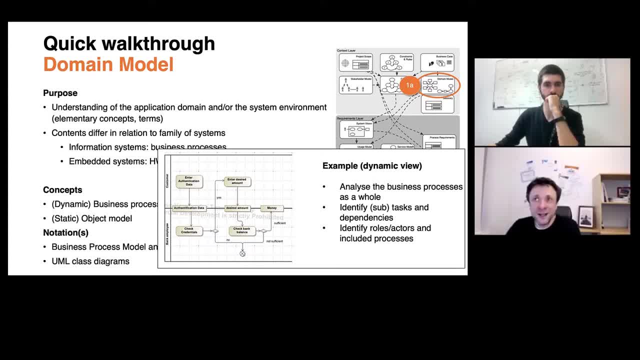 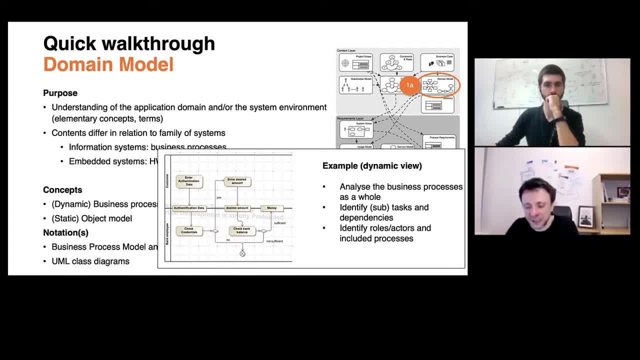 infer the to-be status, the future status. Just take one note with you that if you do it that way, it tends to be an own project. Important is that the domain model captures the intended status, the to-be status, the idealized view on the workflows we would like to have supported. 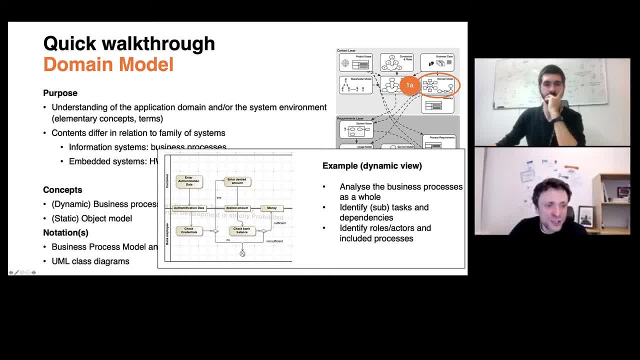 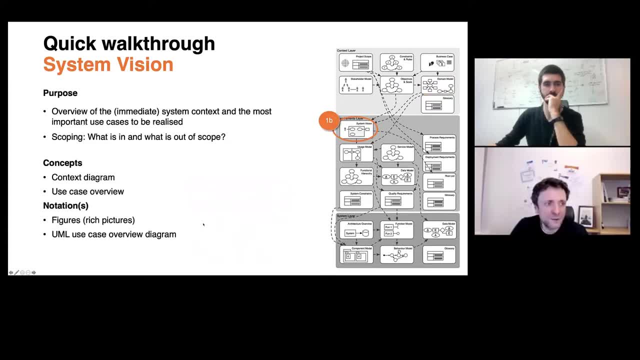 Now, once I have understood which task should be accomplished, I can start thinking about my system vision. Now, the system vision fulfills essentially two purposes. Number one is to provide an overview of the immediate system context. So I want to define my system boundaries: What is inside and what is outside, and the most. 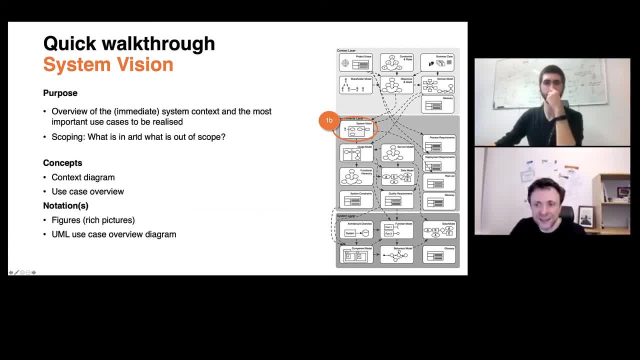 important use cases to be realized. As I mentioned earlier, the system vision is an excellent means to scope our overall project by saying what is inside and what is outside. So I want to define what will be part of my software system and what is not part of that software system. And again, I 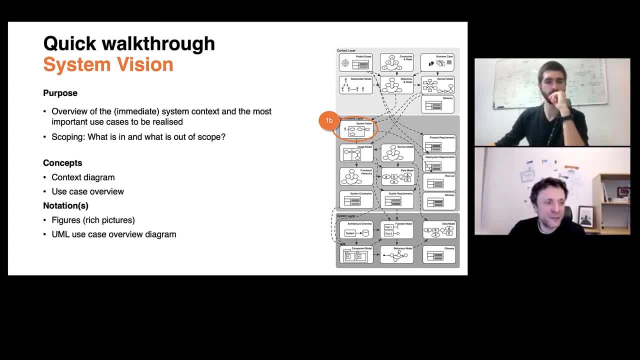 can have two different views on my system vision. One is focusing more on the context and the other one is more focusing on a big picture of the key functionality that I want to offer with my software system, Typically captured by a what we call use case overview diagram. So what you can, 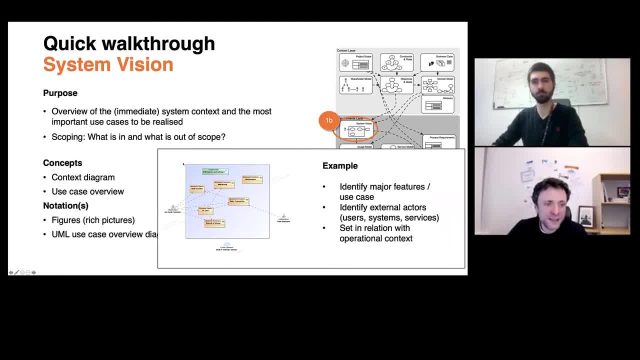 see. here is a more context view. Important is that I outline my boundaries of my software system and the relation to the operational context Can be actors in the form of human beings. It can be actors in the form of external software systems And I outline key features that I want to offer, that I want to provide with my future. 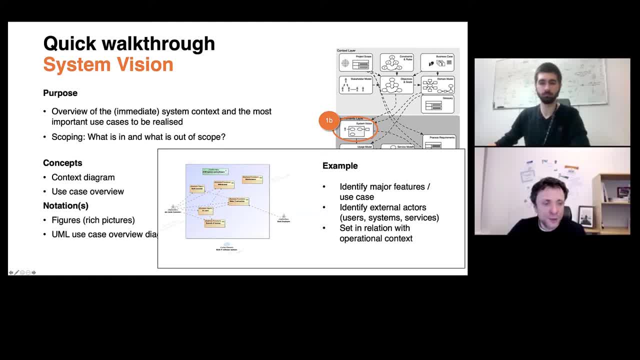 software system, Some of which are in direct relation to my external operational context, Others maybe not. Now, once I have understood those major features, those major uses, I can start thinking about my system vision. So I want to define my system vision. 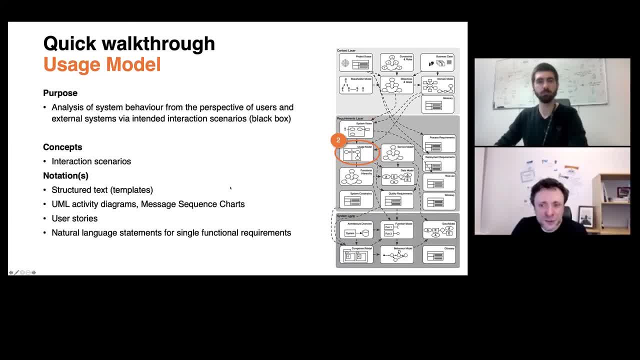 And in the use cases I can infer my usage model. So the usage model I use to analyze the system behavior from the perspective of my external users. It can be human beings or external systems via intended interaction scenarios. Which means that for every single use case that I identify in 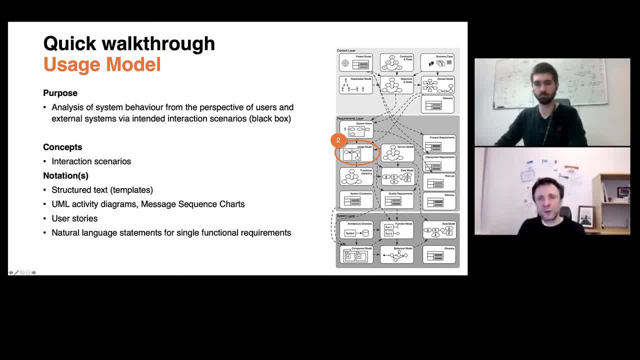 my system vision, I infer how I want to realize these use case in the form of interaction scenarios. So again, we have different concepts here at our disposal. Sometimes I can specify my use cases with structured text, with templates. I can use them. I can use interaction models, proper models for my interaction diagrams. 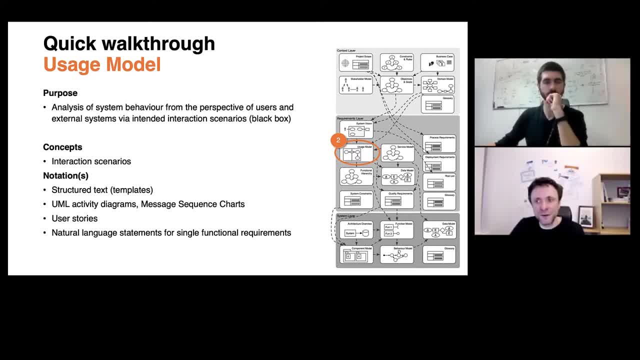 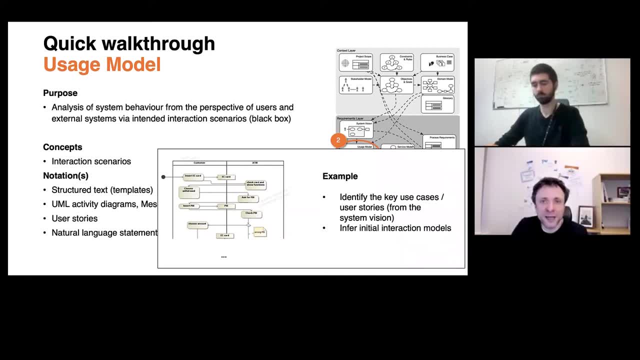 I can use also user stories and so on and so forth. How exactly, we will be discussing later. What you can see here is an example for a human activity diagram that captures how I, as an end user, intend to interact with my ATM in order to 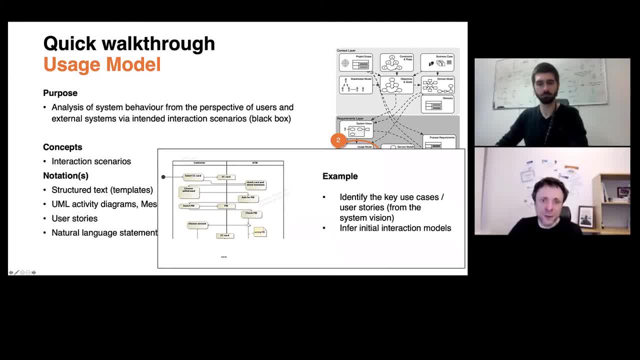 realize the use case I've provided in the system vision, But, more importantly, in order to realize my general workflows in the domain model, the task that I have understood before that. So, for example, I can describe here how I, as an end user, intend to authenticate with. 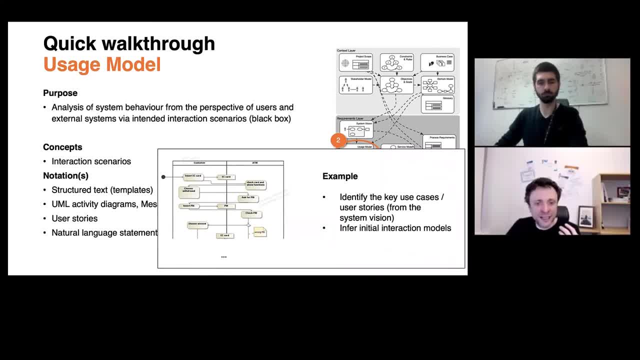 a software system by using my debit card and a PIN. This is the point where I really start taking the black box perspective on my system vision. Once I have understood how I intend to interact with the software system, I can identify the first major functions in my software system, which brings me to the last step. 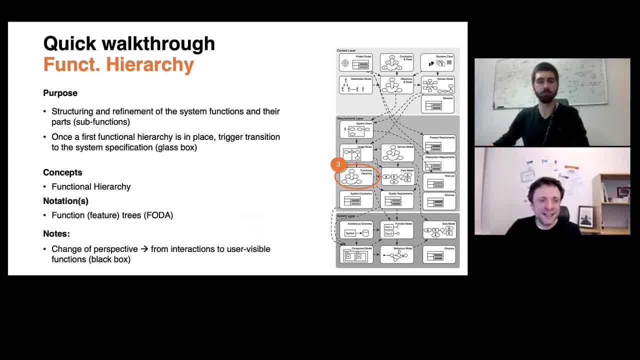 which is the functional hierarchy. Now, the functional hierarchy takes those system-sided functions and does nothing else than a change of perspective. So, for example, in context of a use case where I authenticate as an end user, one element in my activity diagram could be that the system should verify my identity. Now, in my function hierarchy, 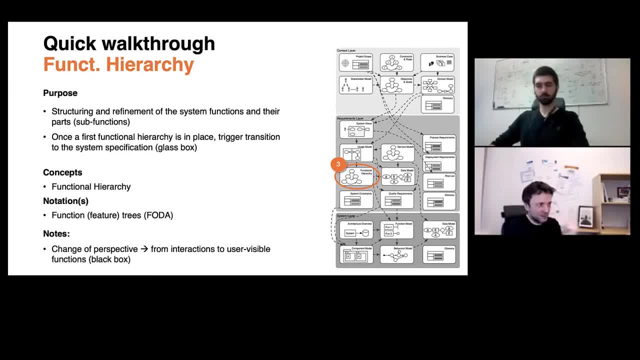 I just leave the perspective of my end user on this system-sided activity and take the perspective of my software system and think about which functions do I need to provide user verification? for example, Instead of saying verify user, I turned it into a function called user verification. This change of perspective. 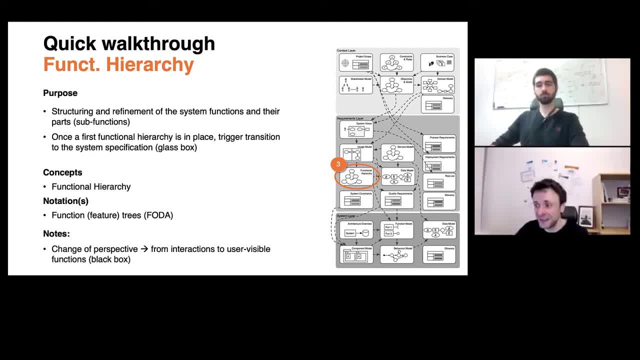 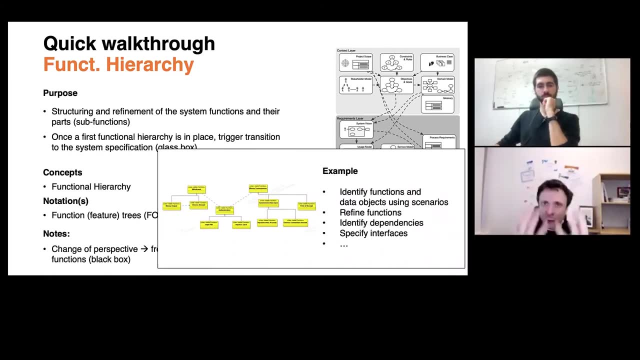 is the change of perspective and the roles in our engineering process. This is the change of perspective from a requirements engineer to my software architect And this is the way how I start my transition into the solution space, by inferring a functional hierarchy, which you can see here at an example, a simple example. I decompose it. 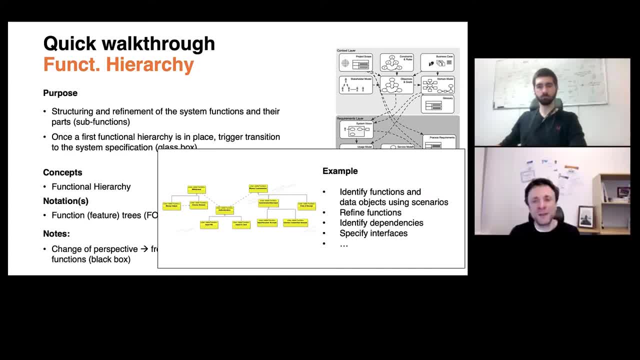 into further sub functions. I start thinking about what the typical interfaces might be: the static interfaces talking about data types, semantic interfaces talking about more detailed interactions, the logical component and architecture, and so on and so forth. So this is the last time we 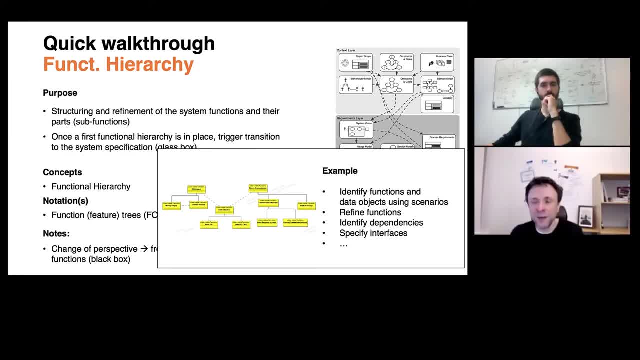 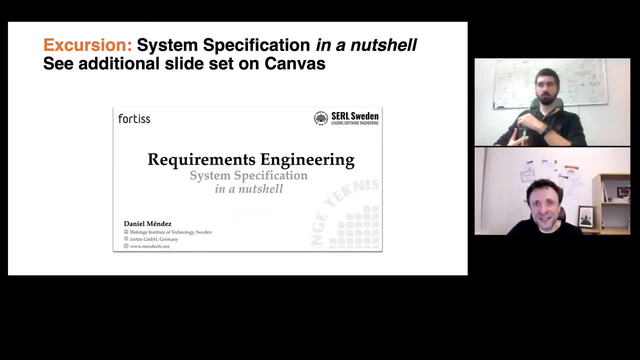 will be talking about functional hierarchies, because they are clearly in scope of fostering the transition into the solution space. It's good to have heard what it is, but it's outside of the scope of this course. Now, in this context, I've created a small additional slide set. It's an excursion because I want you. 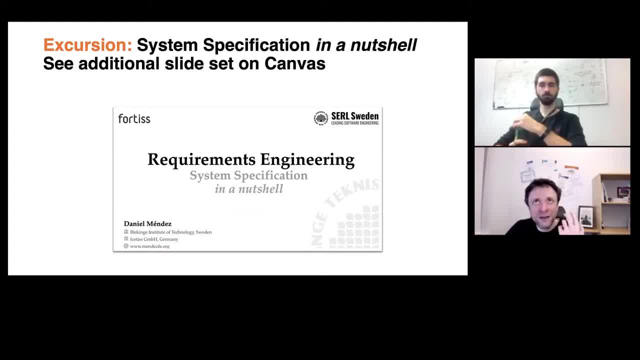 to have at least the opportunity to look into how to do this transition from the requirements specification into architectural design, how these things fit to each other, how the general notion of a component or an interface relates to what we specify in requirements engineering. But again, take this more as 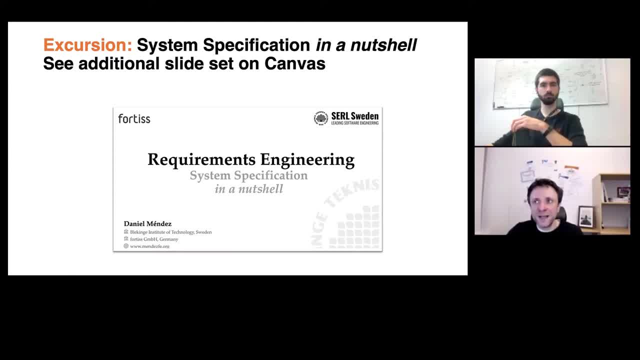 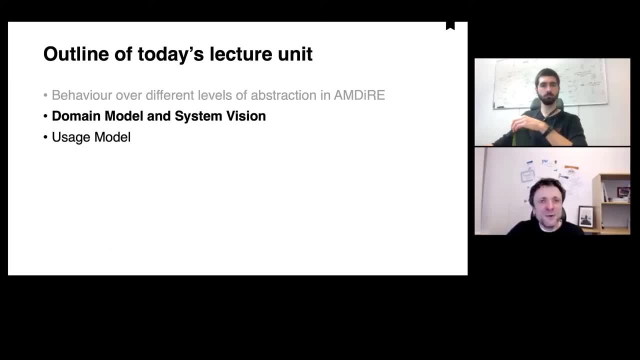 an outlook into what to consider in the design activities, which is clearly in scope of other courses. Now let's move on to the actual content items. So most of the things I'm telling you now in a second will come at no real surprise to you, But still, let's look into into these content items and think. 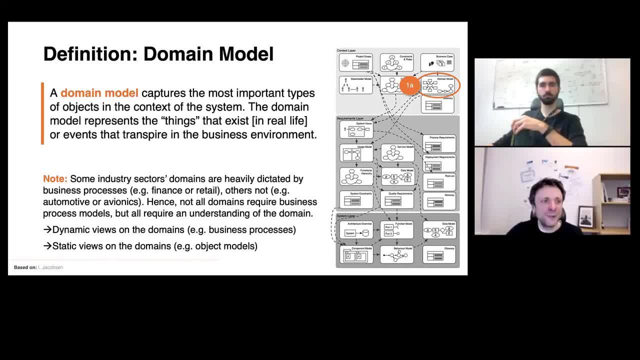 about what to specify, And let's start again with the domain model. Now, what is the definition of a domain model? A domain model captures the most important types of objects and the context of the system. It represents the things that exist in real life. the things that exist or the events that transpire in the 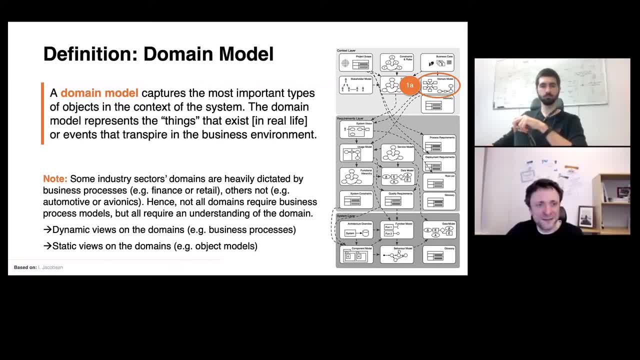 business environment. So reflected by this definition are already the two complementary perspectives I can take on my domain. As I mentioned earlier, some of the domains are heavily dictated by business processes, by workflows, by tasks I need to achieve. This is what you tend to find, for example, in the finance. 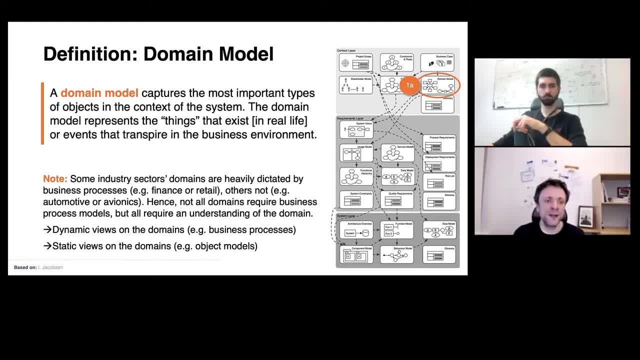 sector, or the retail sector, which we take as a running example here, and others rather not. These others are more dictated by static views, by objects that I might have, by sensors, for example, by bus systems, by more infrastructure related perspectives. Now, what is important? It's important to 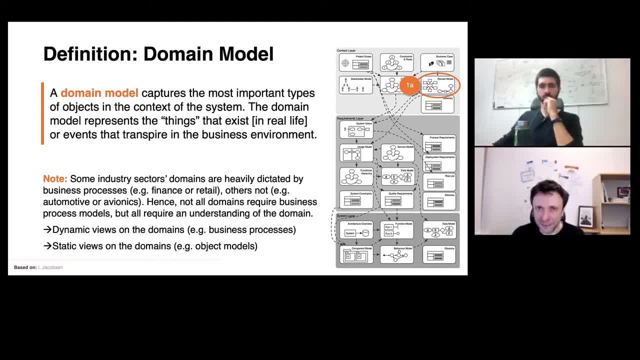 understand that not all domains are the same, not all domains are represented the same way, but all domains require the same level of dedication to understanding the domains, And this is in scope of the domain model. Now let's consider just two simple examples. first, on the dynamic: 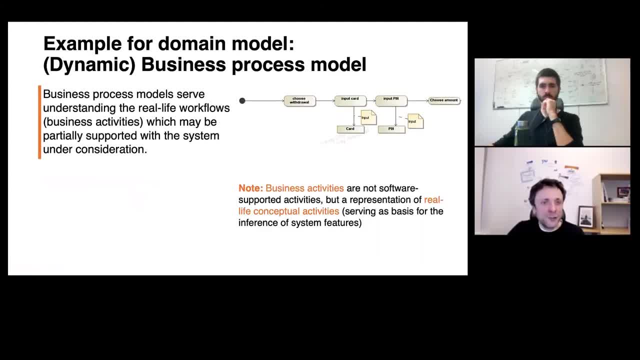 view and then on the static view. What you can see here is a business process model, capturing a more dynamic view on my domain. A business process serves the understanding of real-life workflows which may or may not be partially supported by the system under consideration Here. it becomes already clear that when I capture my 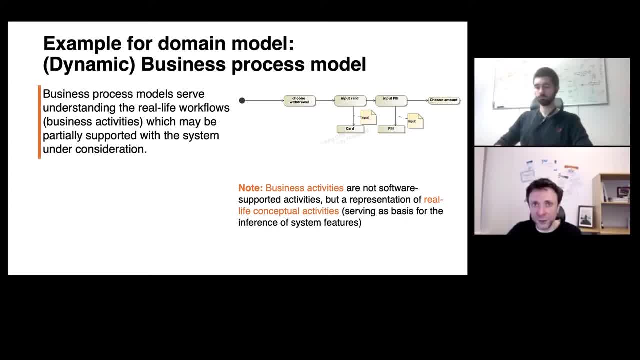 understanding in a domain model of the workflows. I might want to support that. not everything that I will model will be in scope of a software system. More importantly, when I capture these workflows, I focus really on the essence, on my understanding about those workflows, but I do not yet at this. 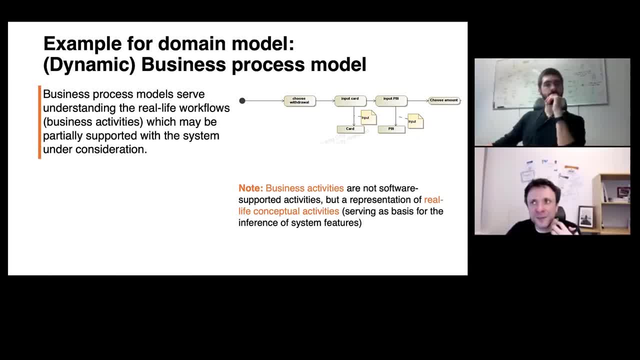 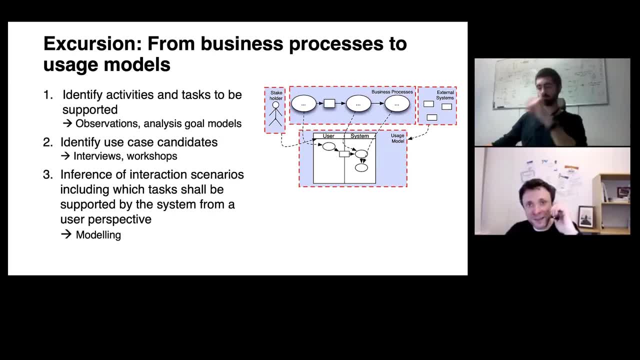 level, specify how my software system is intended to be used in this context. This is in scope of the usage model. So, after specifying my domain model and after inferring my system vision, this is what I model in my usage model, And I do this in a couple of steps, As I mentioned earlier. the first step is really to understand. 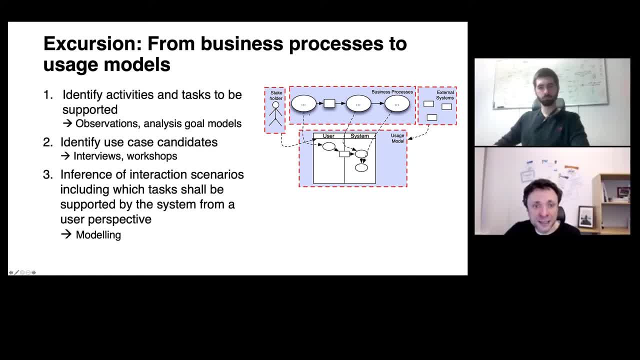 what those workflows are. I identify the major activities that are carried out in a bank, for example, the information that is passed from one activity to the other, and so on and so forth. For example, what information I need to open a bank account. 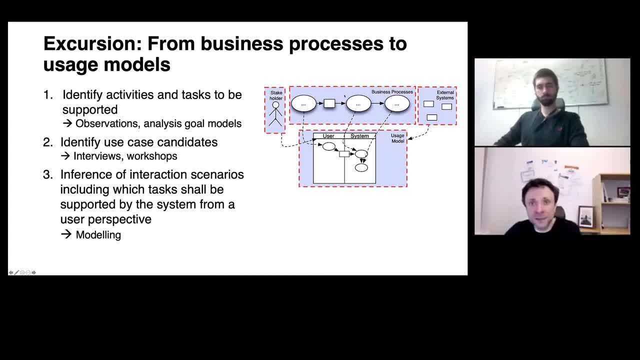 what information I might get from a user or a customer in order to open my bank account, And I can do this in a couple of steps. I do this in a couple of steps. As I mentioned earlier, do this typically by doing observational studies, but very often you find these descriptions already. 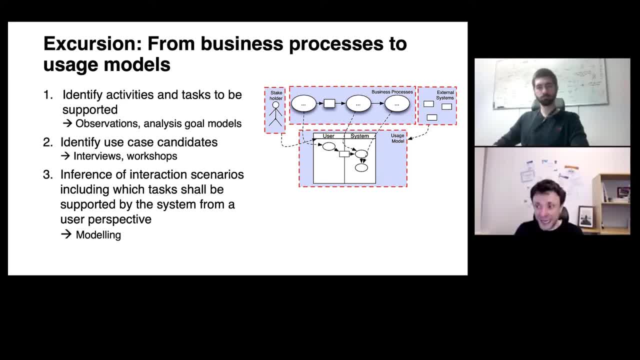 in organizational documents that capture the very essence of their workflows, that specify the rules of the domain, the business rules that need to be applied, For example, how to calculate interest rates. All these information are typically- at least for larger organizations- are typically captured already in reference documents. Now, in a second step, when elaborating 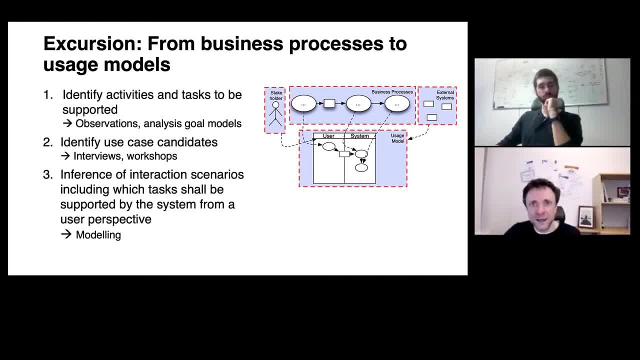 the system vision I identify what we call candidates for use cases. So I think about which of the workflow elements or which of the excerpts in my workflow I might want to support with my software system, And in a third step I specify how I want those workflows to be. 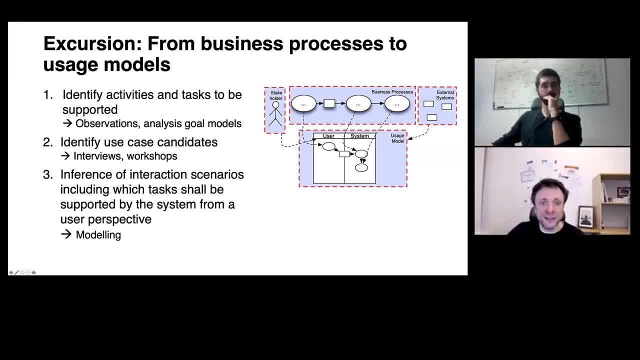 supported by using my software system, And I do this via the software system, And I do this via the software system, And I do this via the software system interaction models. So I say, for example, which of the tasks should be done by the end user. 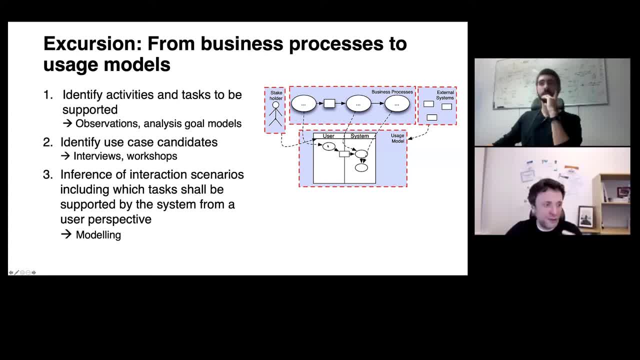 for example, when registering or opening a bank account using a web-based application. So what is what the end user has to do, What is the information that he has to enter in my software system And what are the tasks that remain in the software system? So, for example, how do I identify? 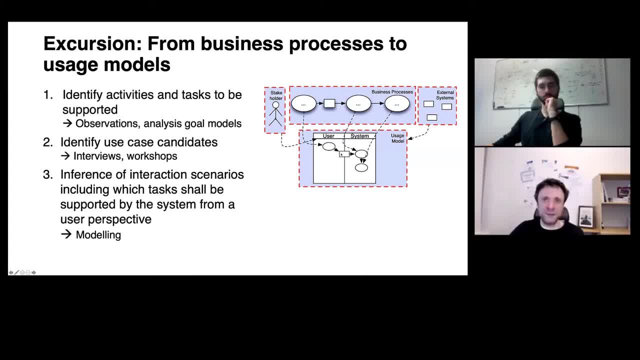 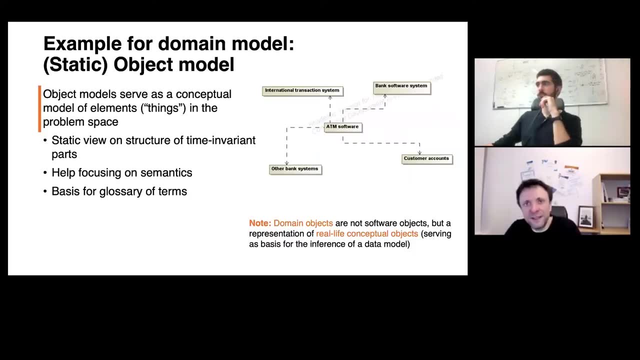 myself. How do I specify my bank ID, for example? This is in scope of the usage model And this is in scope of the modeling activities that I tend to do when conducting my requirements analysis. Okay, Now let's focus on the, at least briefly, on the static perspective. The static perspective. 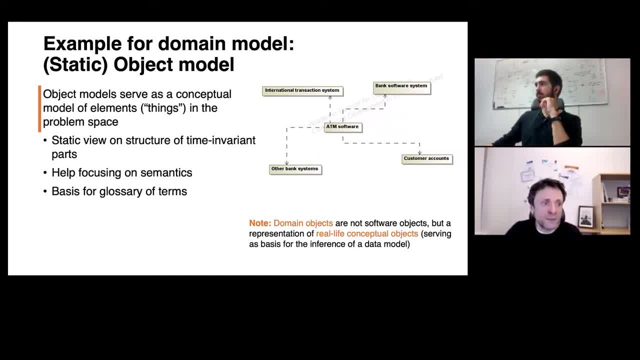 captures or is represented by an object model that serves as a conceptual model of the elements, the things that are important in my problem space, the things that have a certain relevance to the business domain, for example. Let's stay still at the example of a banking sector. 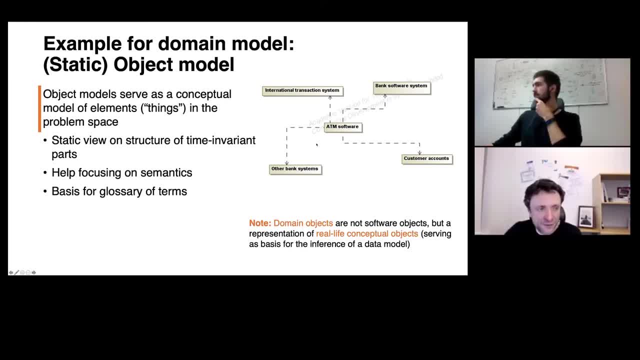 in mind, In my object model or in my static view. I typically focus more on the elements that might be important, the information elements that are important, and the proper meaning, the semantics. For example, I can specify what a bank account or a customer account consists of. 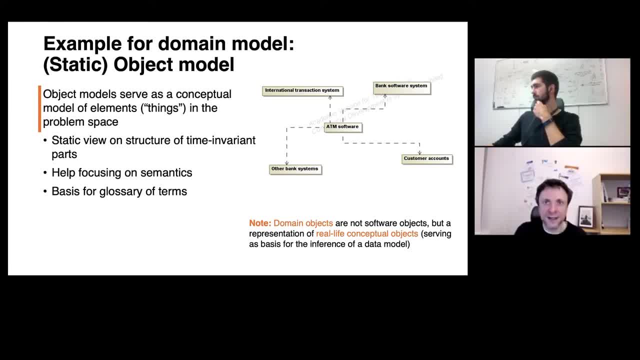 What is the information that my bank needs in order to process opening a bank account? But again, same as with the business process models, I do not focus on how I might want to use my software system, but rather what the business process models are So I can specify what a bank account. 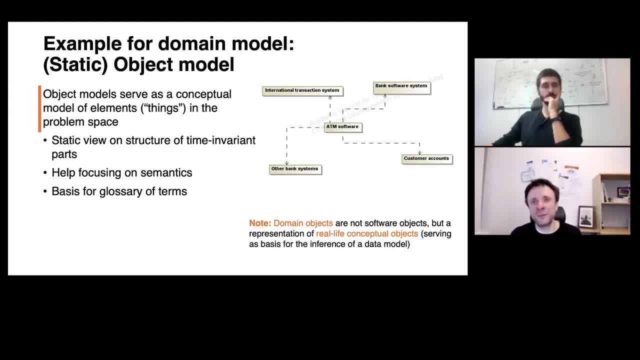 or an account. lots might be and what not. For example, if I have an account that I want to use during the vidae period, I can specify which of these elements might be and some of which might be later represented in my data model, others maybe not. This is a decision I take. 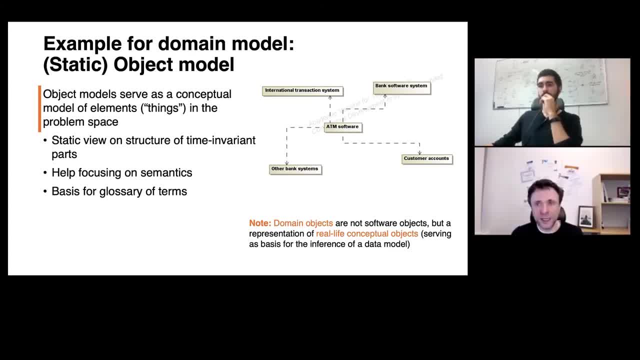 Later. Not all domain models need to be captured via a proper model. as you can see here, Very often you can achieve very good results by capturing the most important elements of the domain In a spreadsheet, for example, capturing a glossary that explains really which elements. 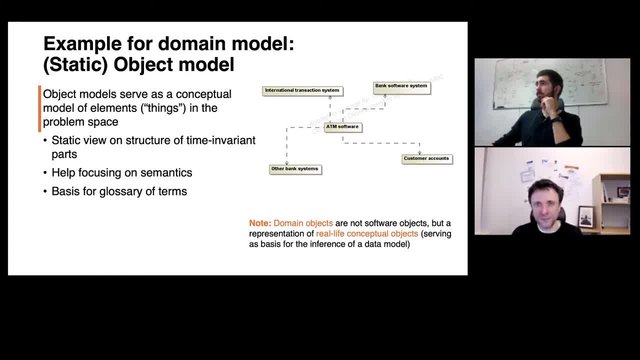 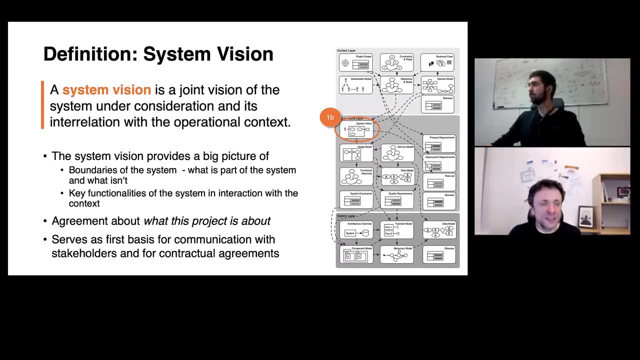 are in scope of a object model in which not- And here again we focus always on the essence, those things that are really important to understand the actual domain, the operational context. Now a couple of words on my system vision. So the system vision is a joint vision of the system under consideration and its interrelation with the operational context. 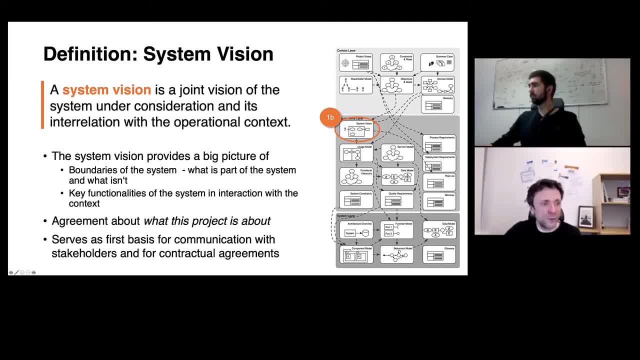 Again, I focus on two things: I want to understand what the boundaries of the software system are, So what is inside of my project and what is outside of my project, And I specify what the key functionalities of my software system are in interaction with its context. 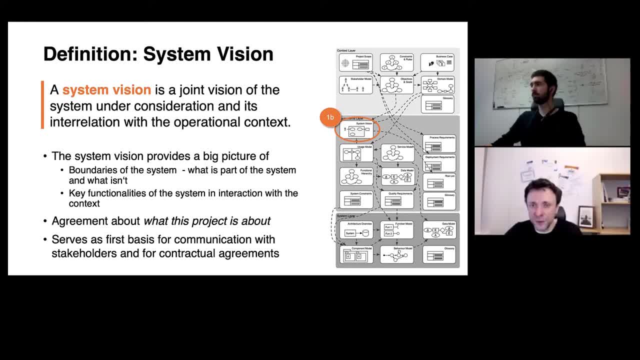 I specify what the elementary use cases are that I want to support with my software system. Keep in mind: the system vision is the entry point into the software requirement specification and is the ultimate means for communication and scoping, And very often it's part of an agreement and even a legal agreement. 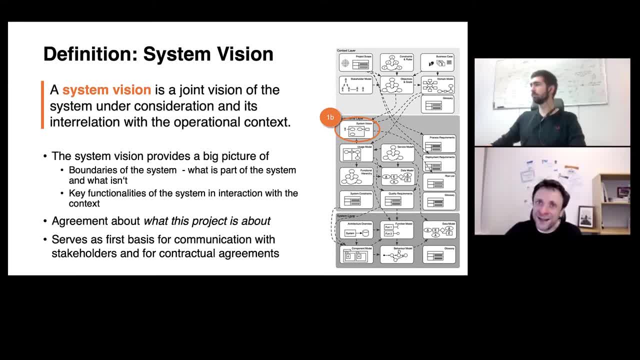 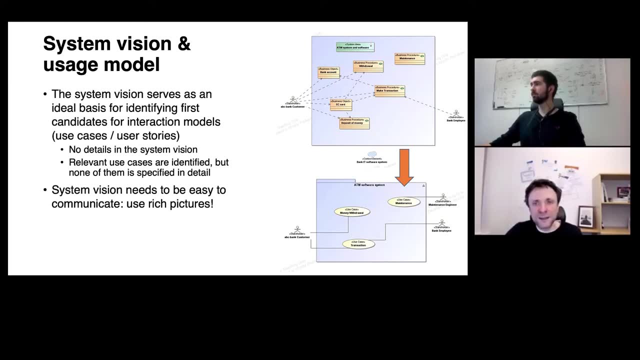 So you will find one way or the other, represented in one way or the other, a system vision as part of the contracts that specify what to do in an engineering project. Now, what you can see here is the relationship between the system model and the key features that I want to specify in my usage model. 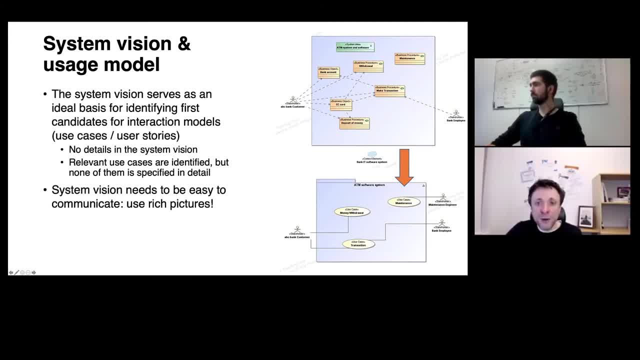 The upper view focuses more on the boundaries and the relationship to the operational context. The lower one is, which you know as a use case Overview diagram, And you can see here already that many of the ways of representing my system vision might want to use complementary diagrams. 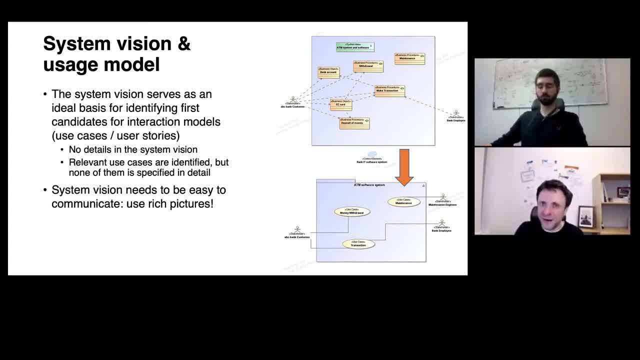 But in some cases we can merge them just to one because they are very, very similar And this very much depends on the complexity of a software system and the project. So if the complexity is low enough and it allows, I can focus just on my use case overview diagram, because it very well represents already the relationship to the operational context. 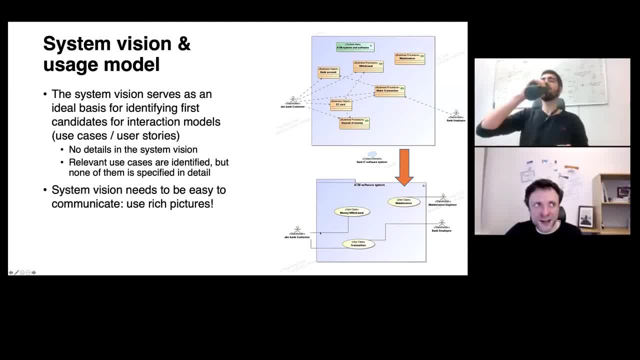 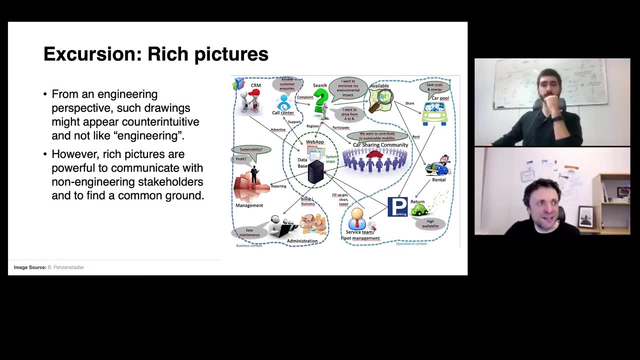 In other cases, however, not. Regardless of how I specify my system vision, important is one thing: It needs to be easy to communicate, which brings me to rich pictures. So what are rich pictures? Rich pictures are a simple drawing of my context and what is inside and what is outside Rich. 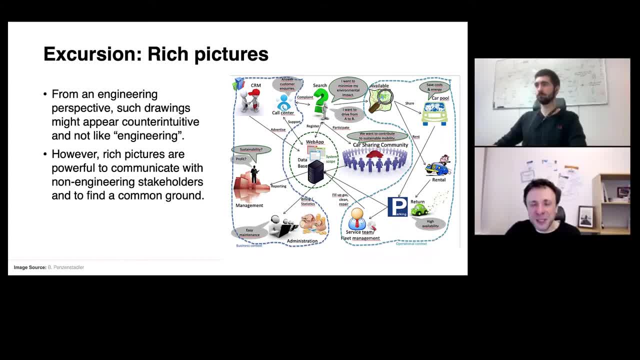 pictures is a perfect way to reduce the complexity, the technical complexity of a system vision. At the same time, rich pictures doesn't really follow specific rules, if I want to say so, specific semantics of specifying this operational context, but it's rather a simple, creative. 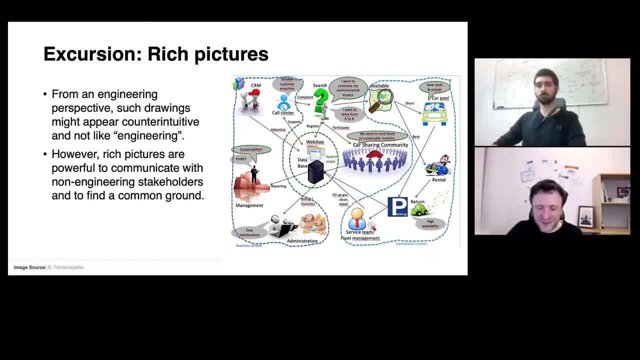 drawing From an engineering perspective. formulating something as a rich picture might be a little bit counterintuitive, but they serve a purpose. They are easy to communicate. When I first saw rich pictures, I should add that I thought that this is really not what we should do in requirements engineering. as an engineering, 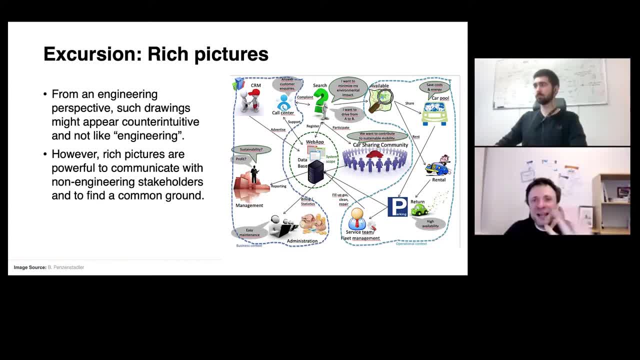 discipline. I was one of those who were propagating the value of goal-oriented requirements, engineering, of using more formalized views, because those formalized views allow us for precision. for statistics, I can model the system behavior In more mathematical terms, in more precise terms, I can simulate those models, but at 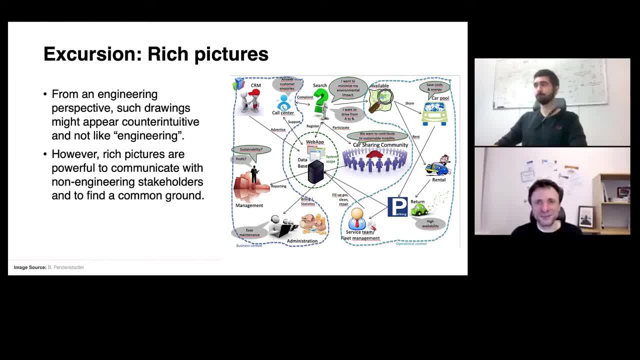 the very end. nobody really understood those models. So I was one of them, thinking like Bob Ross. This is a little bit of an esoteric way of specifying my operational context. Let's prefer more than formalized views. But again I realized. 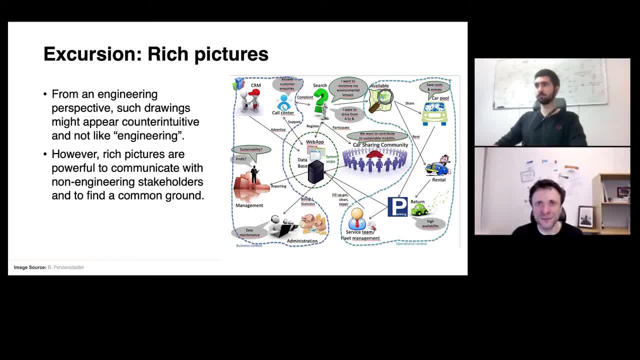 at some point that nobody really understands those complex, formalized views. which brings me to the value of rich pictures, which brings me to the point where I started, rejecting those goal-oriented requirements, engineering approaches, those more formalized views. I can take on my models that might very well be suitable from an engineering perspective. 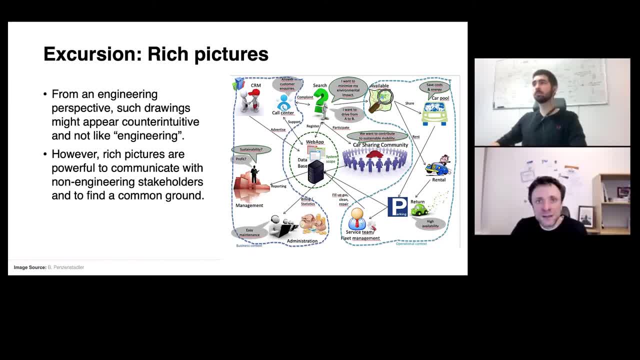 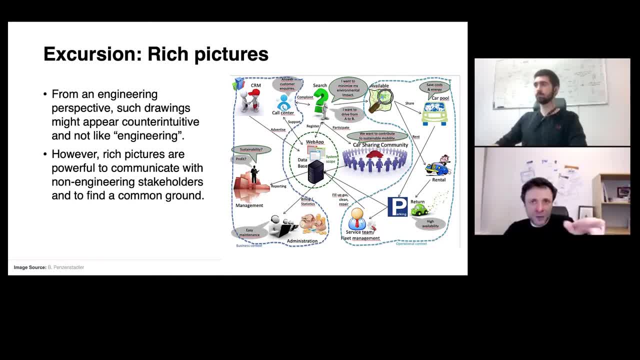 I can locate a free car, I can book it, I run to the car, I take the car, drive through the city, park it somewhere else for the next user to use. And those car sharing applications tend to be rather complex. And in this rich picture I specify essentially three things. 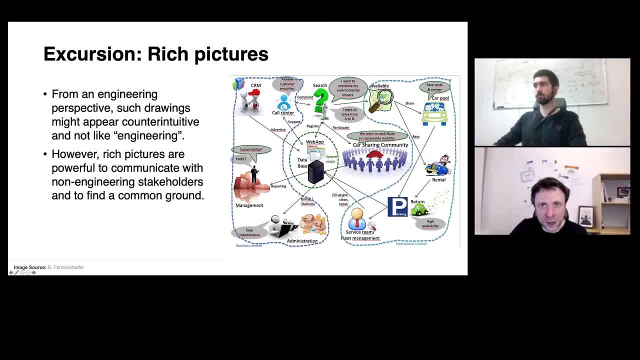